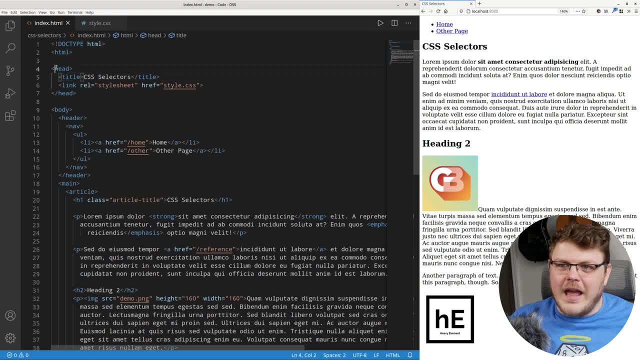 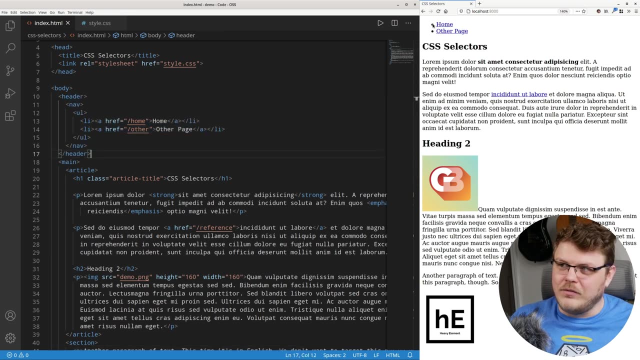 here is HTML. We have our head, where we specify metadata for the document as well as links to items that we need for our stuff. And then we have our body here, And this is going to have our header, which is this list of links to navigate around. And then we have our main tag with an. 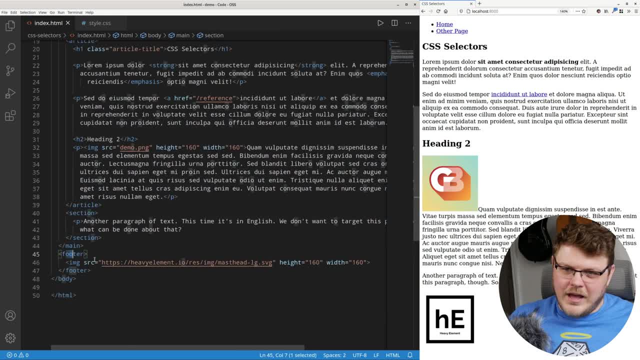 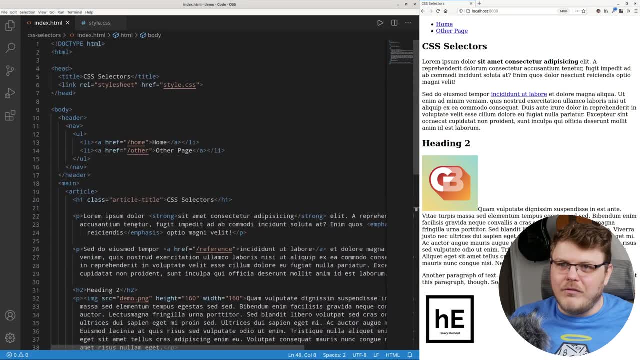 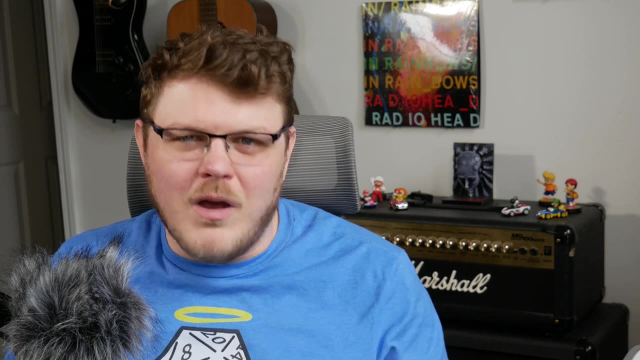 article in it As well as a section, And then we have a footer tag, And you can see here that this is the browser's representation of this document. The second part of the web is going to be JavaScript. JavaScript or, you know, WebAssembly, Some kind of logic that's built into your browser. 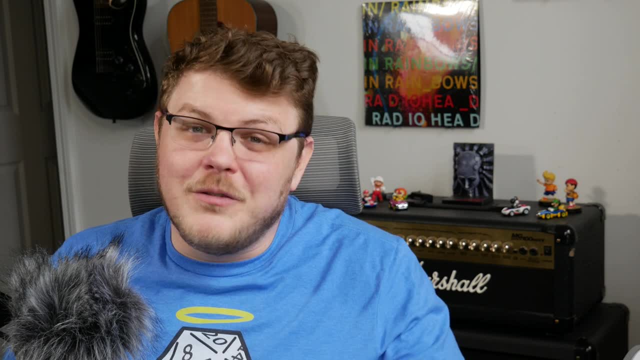 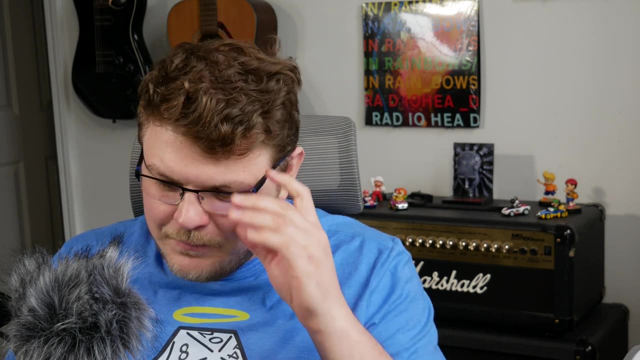 that your browser can execute. We're not going to talk about JavaScript, because we don't need it in this video. The final thing that we need is styles, So cascading styles, CSS. Now, this CSS is empty, because we're going to fill it out together here, And what CSS allows. 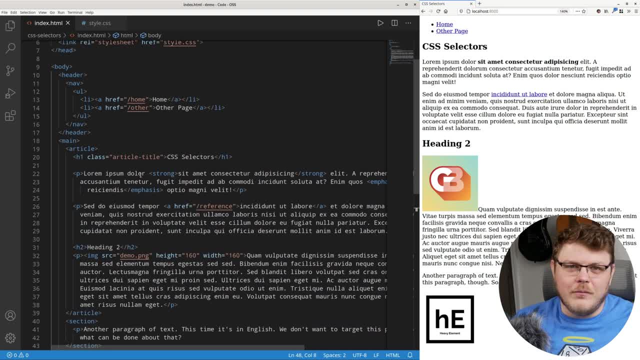 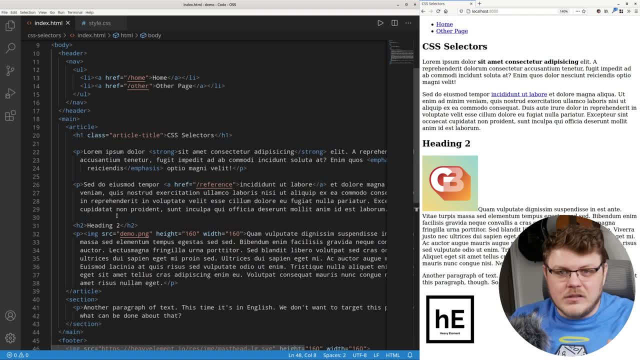 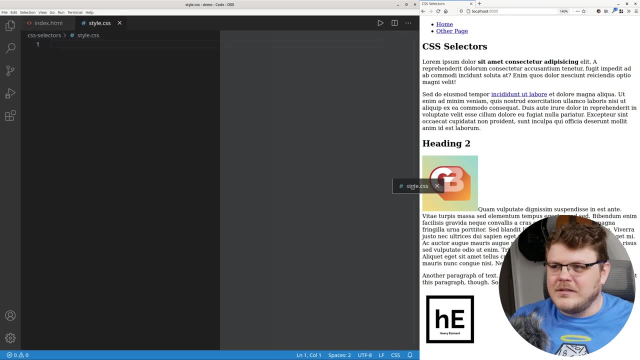 you to do is basically write queries for your HTML document that will be able to then apply styling to those queries that you have. Let's go ahead and do this. Let's start with stylecss. Now you can see we're linking stylecss here in our head. 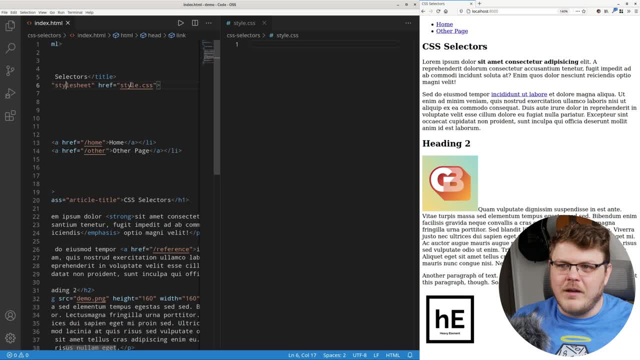 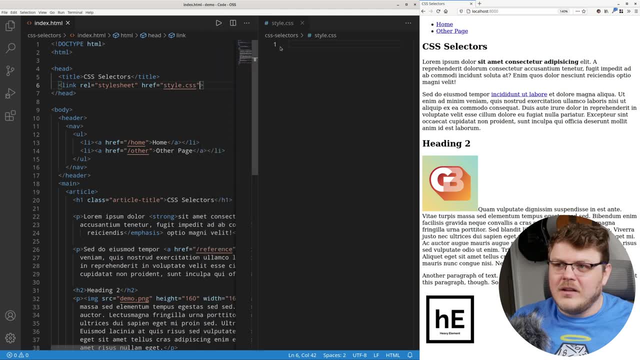 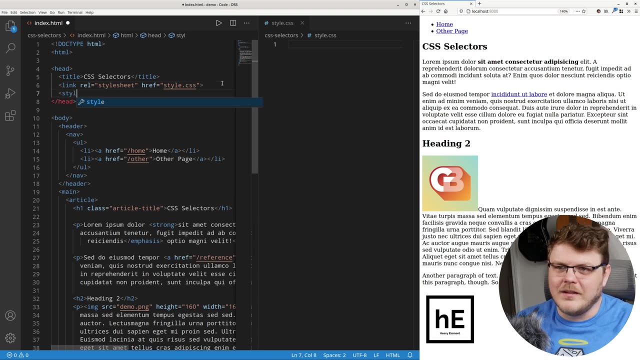 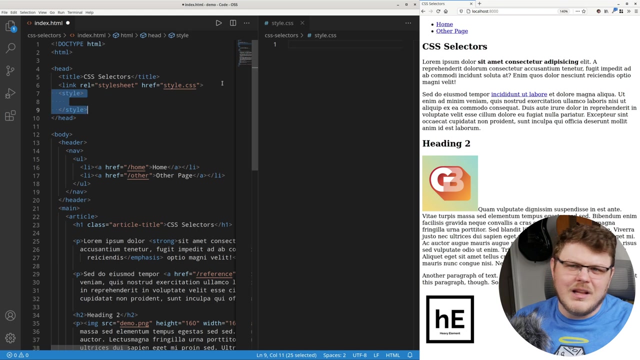 We have link- rel equals stylesheet and href is stylecss, And that's necessary if you want to have your style document included. Now you can do inline styling with a style tag. Wow, I can't type. So if you have a style tag in your document, you can write CSS inline here. But it's cleaner and 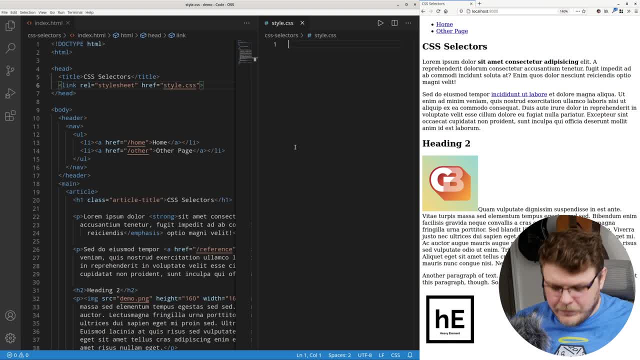 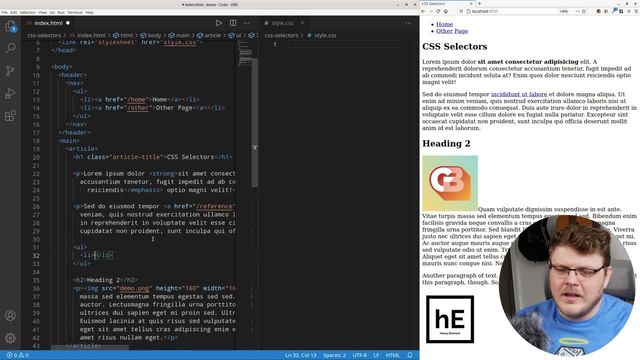 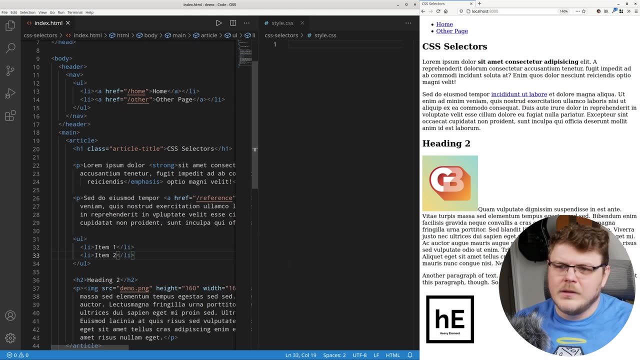 nicer to do it with an external file. Now I wanted to make an unordered list here. So we're going to do li and then we're going to go item one And then let's do item two. And now this is going to be necessary because I want to show. 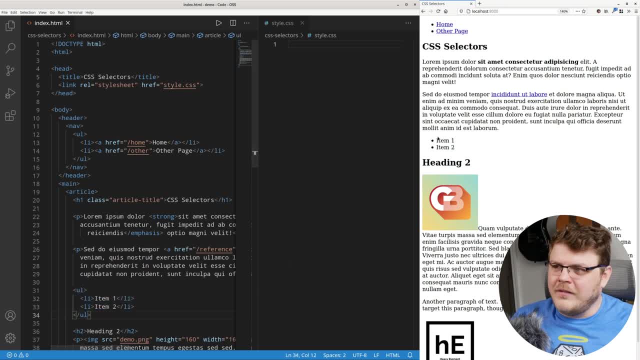 you guys a couple things. So we have our unordered list here and that's right here, And you can see that our navigation bar is actually an unordered list as well. with these bullet points You could do an ordered list which would prepend your list items with numbers. You can also do letters, You can do whatever, But 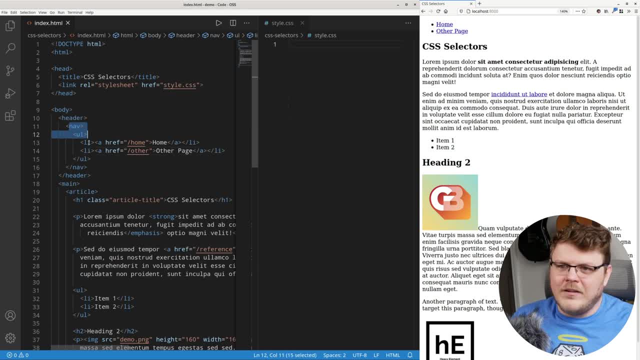 let's go ahead and select our navigation, UL. Now, if you know anything about CSS already, you'll know that you can target items by listing their name here. So we have our selector- is what this is called- and then we're going to have a list of properties inside these. 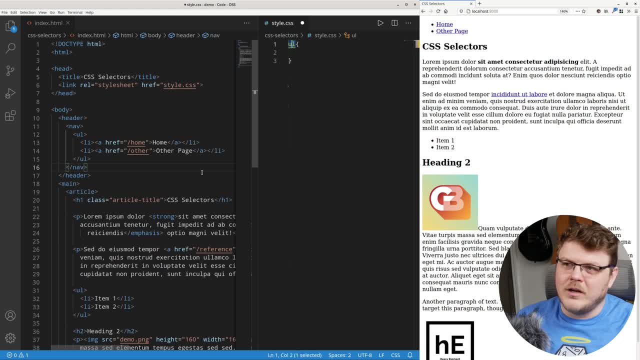 brackets, And so UL is a tacit tag. That's what these are going to say. So here we can also assign a URL, We tag name, so we're going to be matching any tag name: UL. That's what this selector here states. 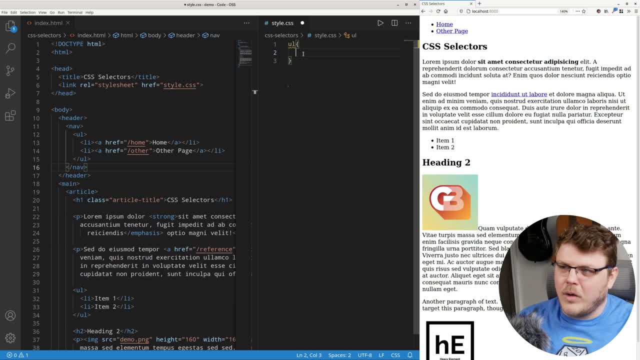 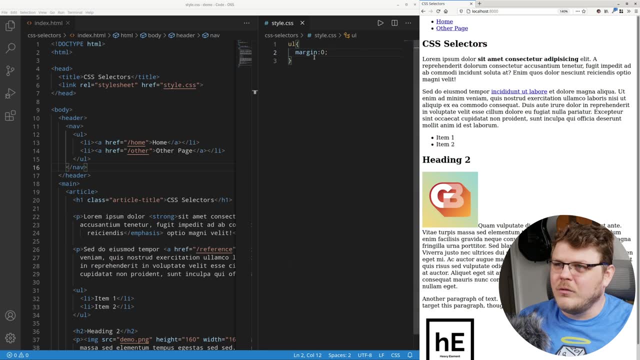 And we can say get rid of the margins here. So let's say margin zero And let's refresh the page and you can see that the margins were removed. We can also do padding, And padding is going to be a bit more of a significant thing. 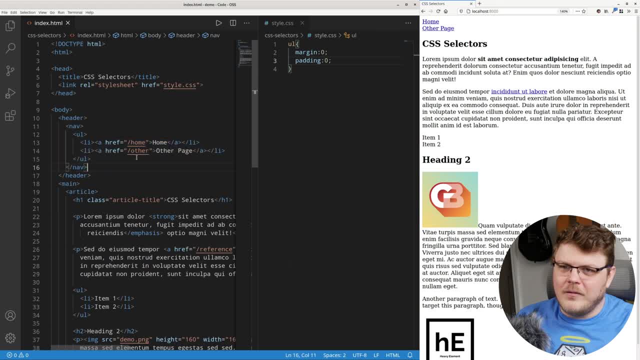 But I said we wanted to target our navigation UL. So one of the nice things about selectors in CSS is that you can actually compound them. So you can do nav space UL and what that will do is it will find any unordered list that is contained within a nav tag. 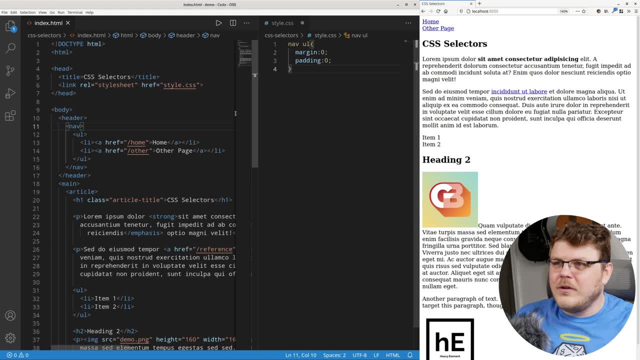 So this one and this one right. So now, if we save this and we refresh, you'll notice that this unordered list won't be affected by what we have done here. So if we refresh, boom, look at that And again we can target the list items in the UL here. 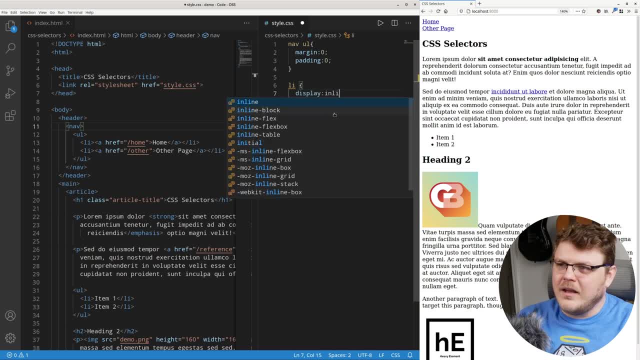 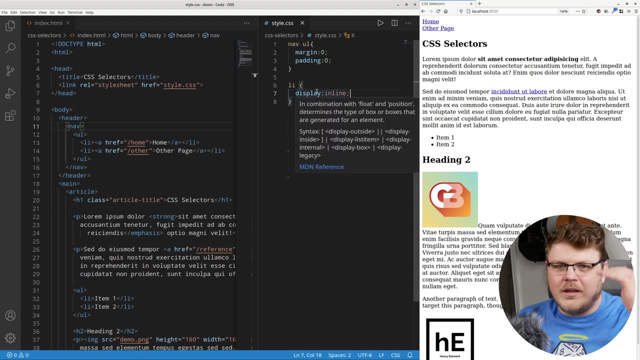 So we can say UL and we can say display inline, And what that's going to do is it's going to make them display in a line rather than breaking to new lines. And there we go. You can see we have home other page. 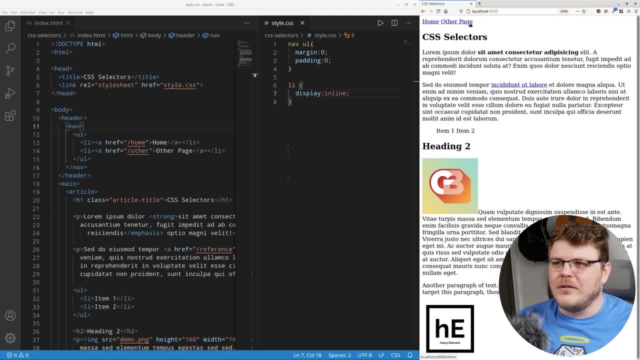 And now it starts to look more like a traditional navigation panel, doesn't it? But you can see? Ha ha, We've also updated this down here. We don't want to update this list, So let's prepend this with a nav. 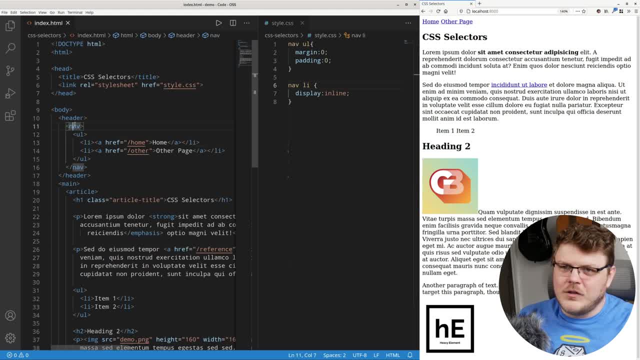 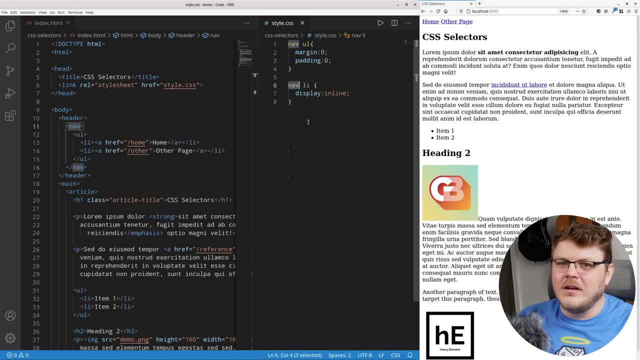 And you can see, even though list item is two layers down from the nav element, these list items are still contained within a nav element, And so that selector matches. Cool, We're starting to figure this out. I hope you're following along. 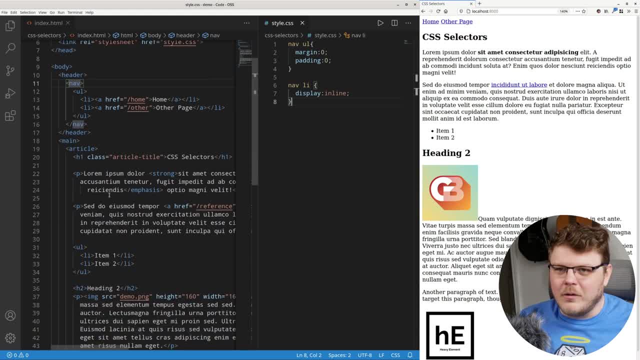 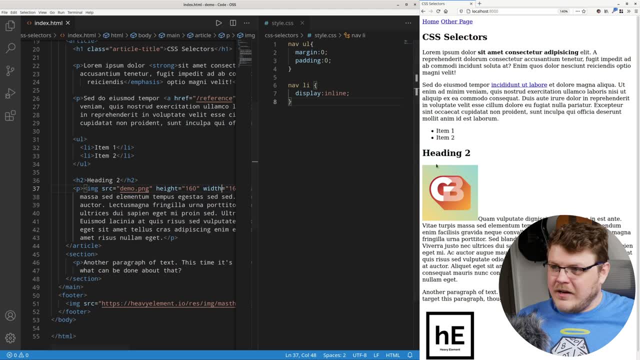 You know I'm going to explain this in a relatively straightforward way, So let's scroll down a little. You can see that we have an image tag And this image tag is represented here under heading two in the paragraph right, Or the P tag. 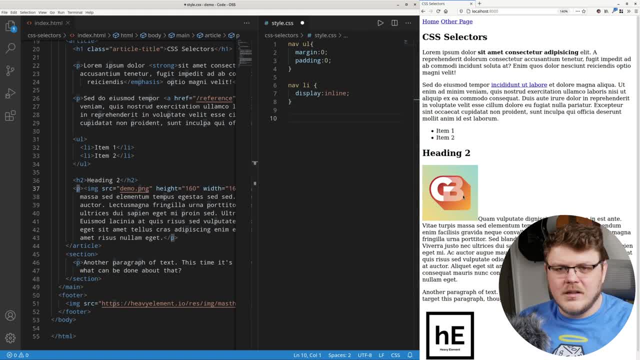 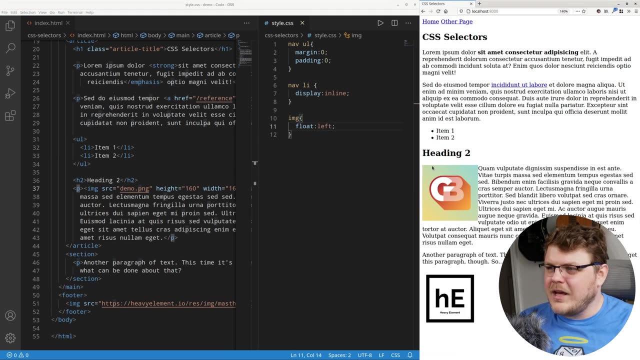 So let's say that we want to have our image tags float around the text and have the text wrap around the image. So what we could do is we could say image And then we could say float left, Okay. And if we hit refresh you can see: hey, we're floating left. 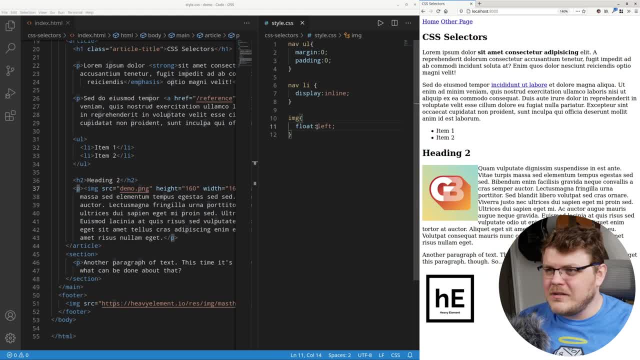 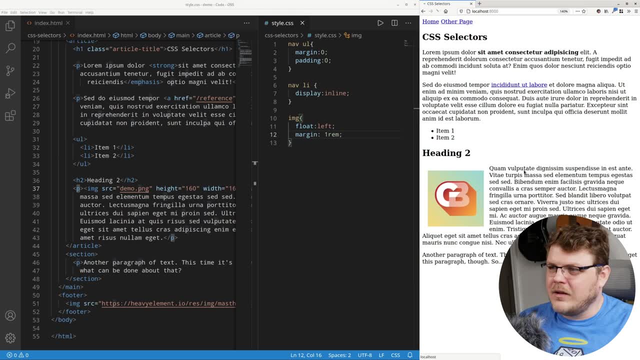 And that looks great. except we want to add a little bit of spacing here, So let's go ahead and add margin. We can just specify one rem, which is a relative unit, And so you can see that we have the space now around our image. 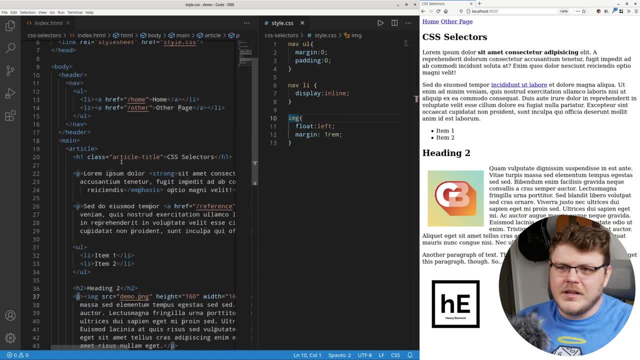 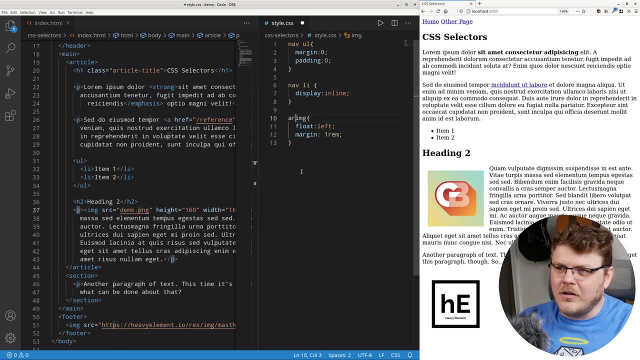 But we're also affecting this image down here, So let's instead look at our HTML. How do we want to select this image? We could say any image that's part of an article. we want to float left and have a margin of one rem. 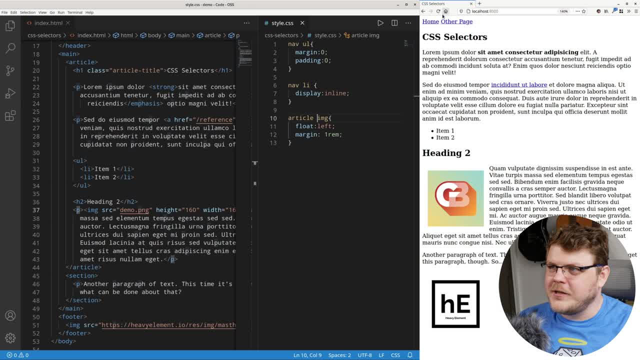 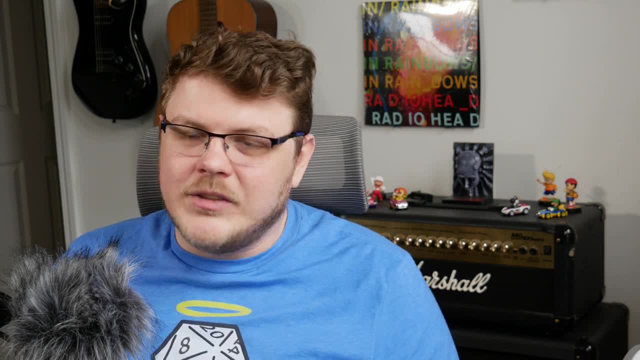 And now, if we refresh the page, this is not going to change, but this will Watch Boop. You see that That's pretty cool. So far, we've just been selecting tag names, which is fine if you want to do that. 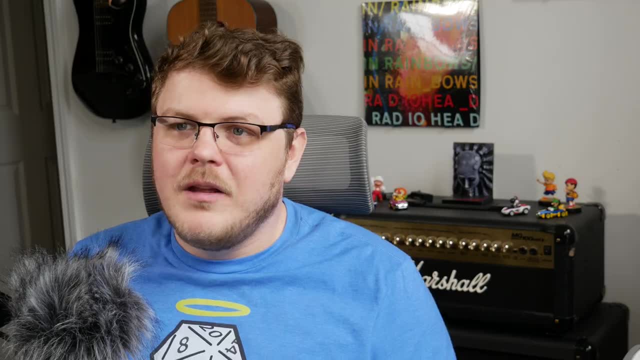 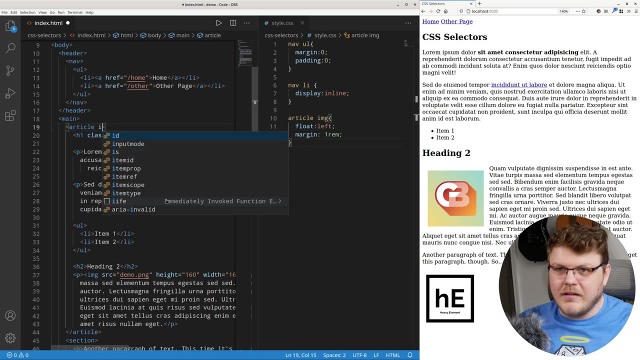 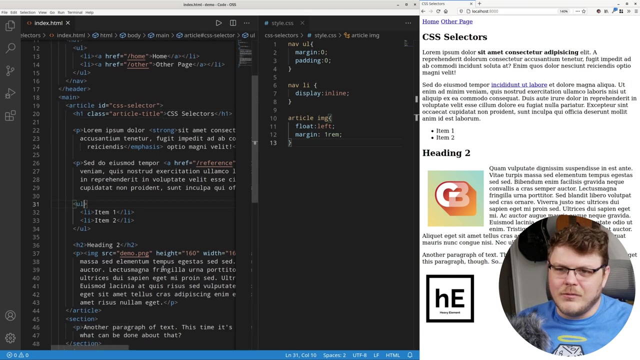 I mean, there's many valid reasons that you would want to do something like that, But You can see here that we have class article title right And you can also have things like IDs, CSS selector And there's all kinds of different things. 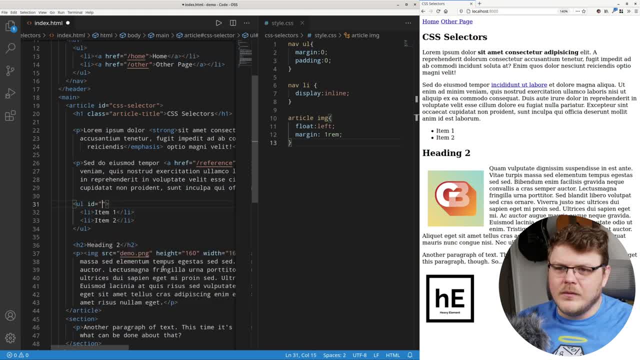 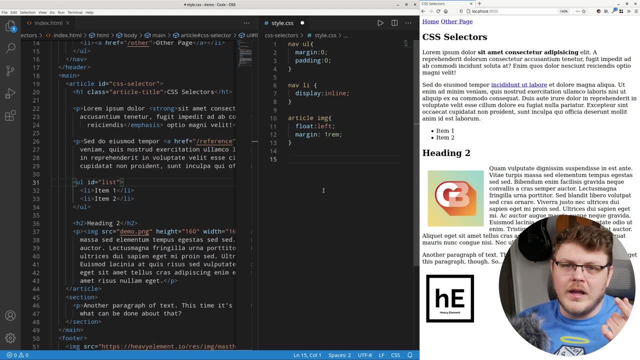 Like we could have like an ID of list, right, And you can actually query for those things. Now, the way you would query for a class is with a dot, So let's say dot article title And now whatever properties here are going to be applied to this H1 tag here. 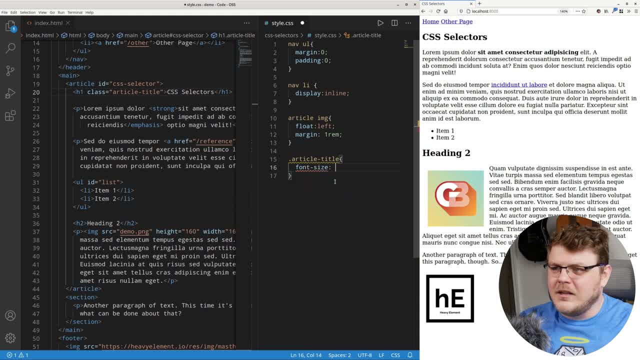 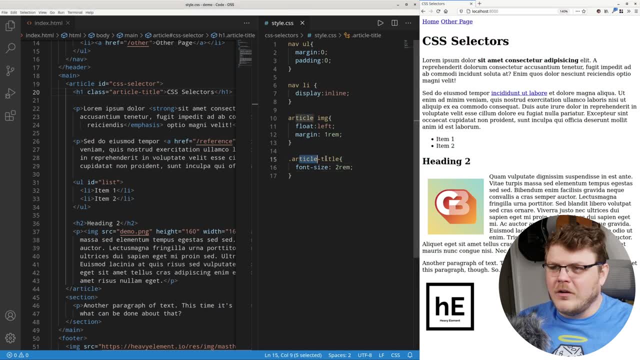 So we could say: font size is two rem. And there you go. So you see, we've increased the size of our article title. here You're able to apply styles by querying for them based on their class name. So let's go over here and let's add a class. 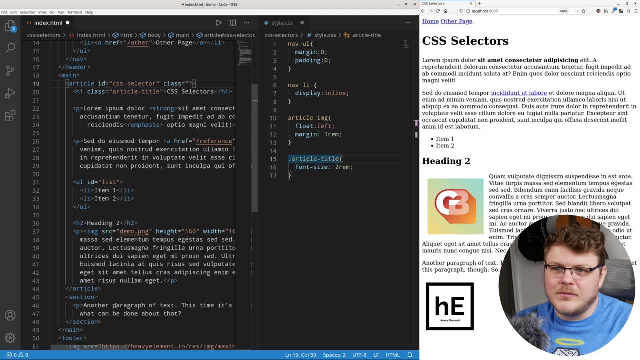 Let's add a class And you can have multiple classes separated by spaces In your HTML. So let's say article, Just give it a name, a class of content, right, And then let's go down here to section and let's also add a class content. 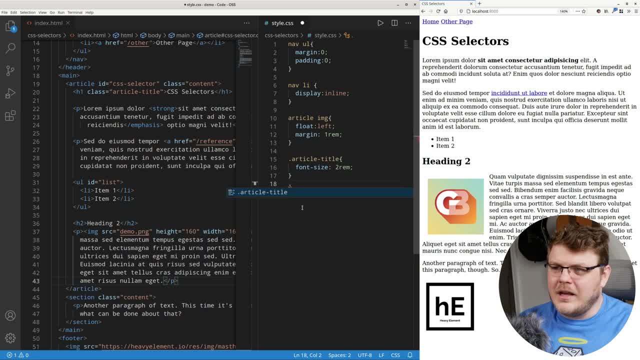 Okay, Now what we could do is we could say content and we could say width, and we're going to say 70%, And then we can say margin zero, Auto. And what this is going to do is this is going to make the this, all the, all this content. 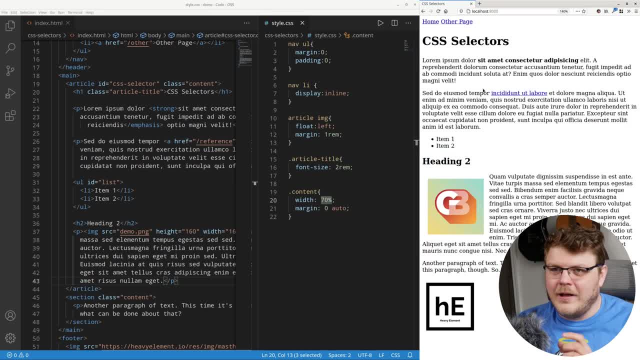 here 70% the width of its parent- In this case the width of its parents- going to be the viewport or the browser window, And then we're going to set the left and right margins to be automatic, So it's going to center itself inside the viewport. 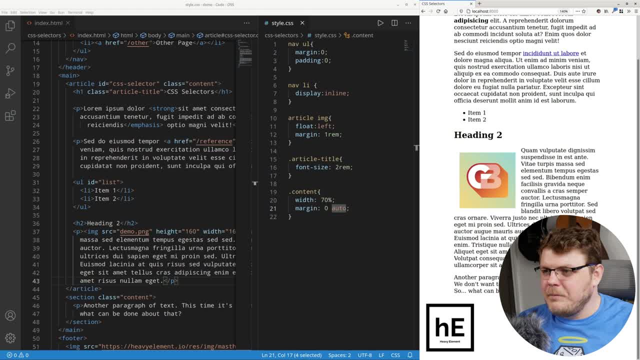 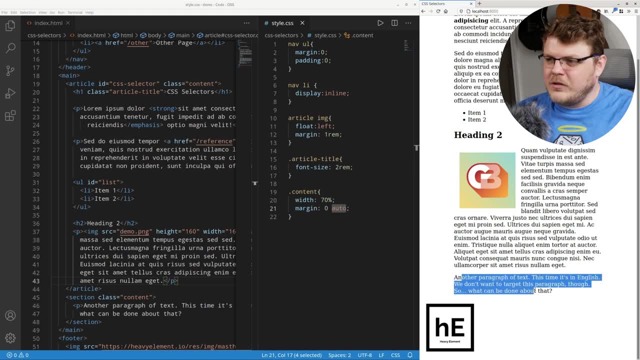 So if we refresh the page, you can see that we we've done that Right, But Okay, So what we can do is we can actually target this. Let's say that. let's say: for some reason we don't want to target another paragraph. 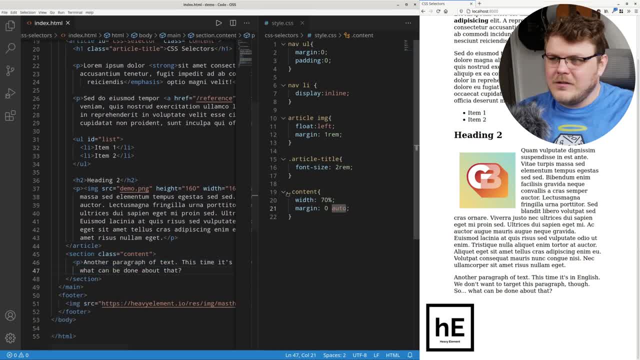 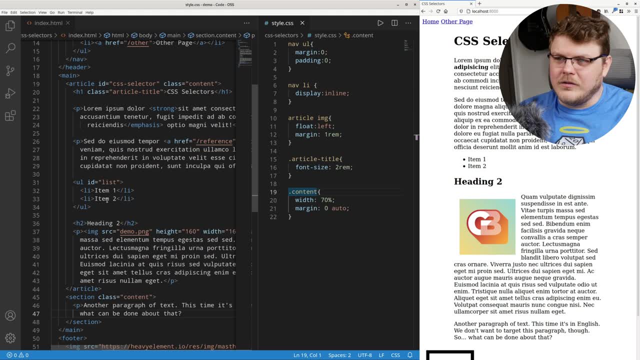 of text. This time it's in English, which is right here. So what we can do is we can actually select for content that is part of an article tag. So let's say article dot content, And so that's going to select for an article tag with the a class of content. 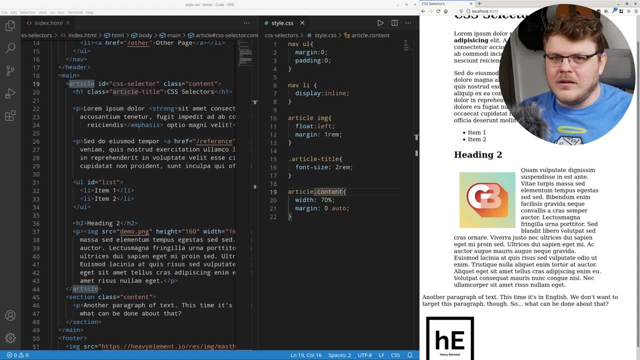 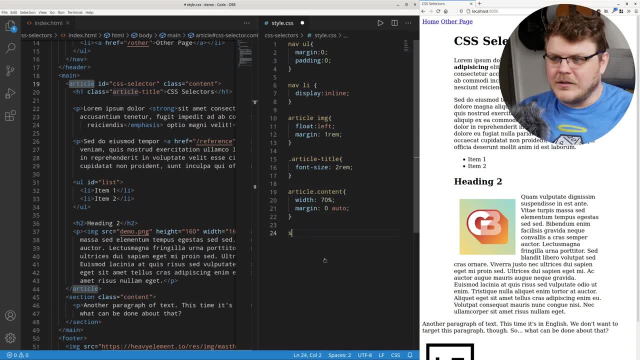 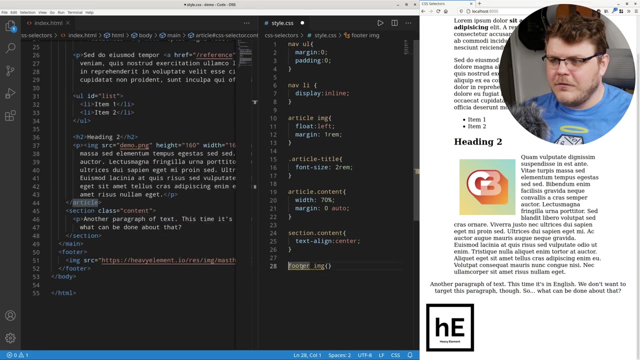 Okay, And you can see now this text is not being centered or or resized, And that's what we were trying to do. Let's say that we want to have our section dot content to be text aligned center, And so now you'll see that this text is actually being center aligned. 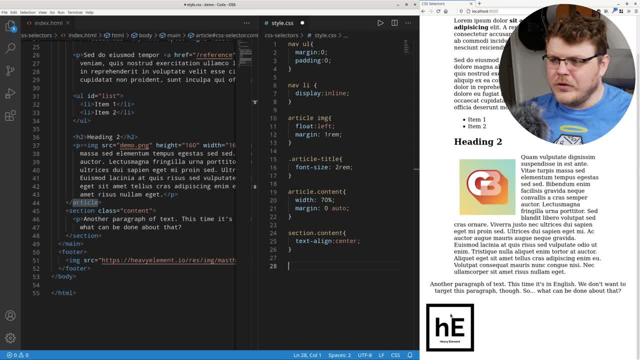 And finally, let's center align the footer logo here. So let's just say footer, Okay, And then we can say text align center and whoops, center, center. There we go And we'll hit refresh, And now you can see that image tags are actually kind of behave like texts. 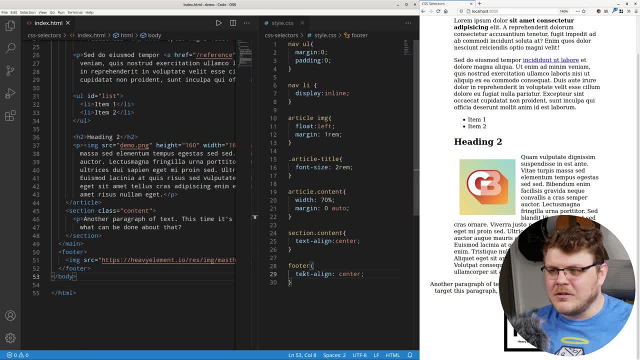 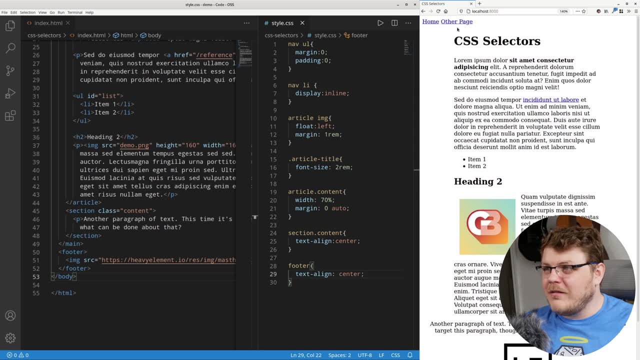 They're in line elements, which means that you can do something like text align, center, and it will, you know, center align it to the parent width. So there we go. We we have a document that's starting to actually look kind of pretty. 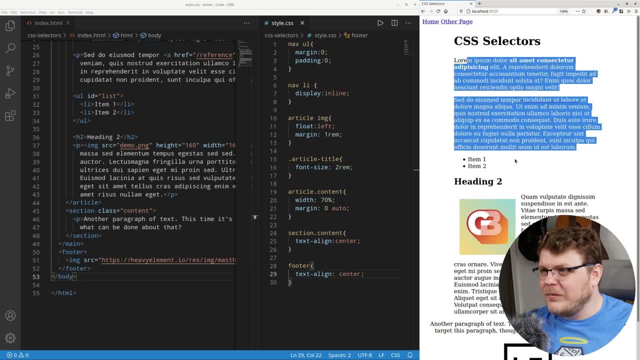 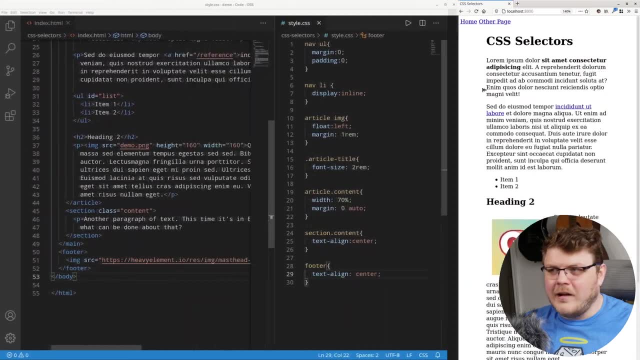 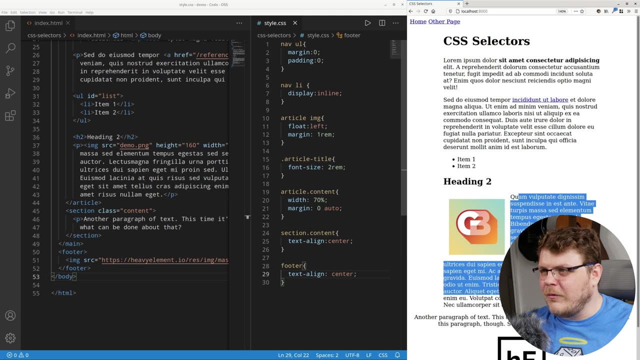 Compared to how it did look. we've got a little bit of you know margins here and we can- actually it'll- resize dynamically based on the width of our window And we have our image floating here and text is wrapping around the image and we have 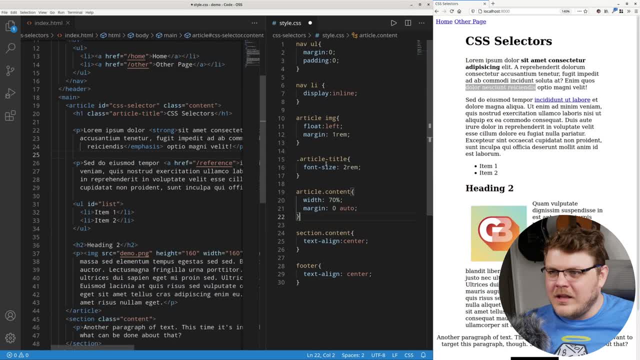 you know our anchor tags. One more thing that I wanted to talk about is that you can actually have multiple classes on an item. Okay, So let's say, for example, another class and we'll just say this is going to be body content. 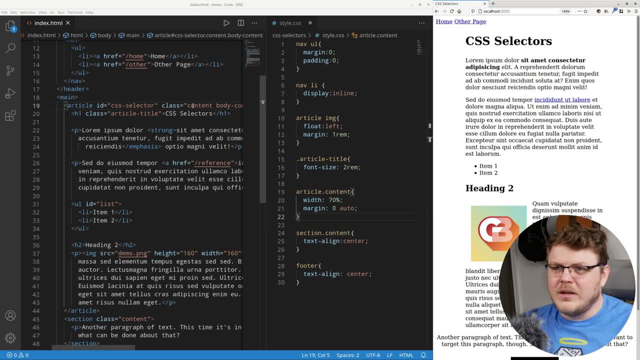 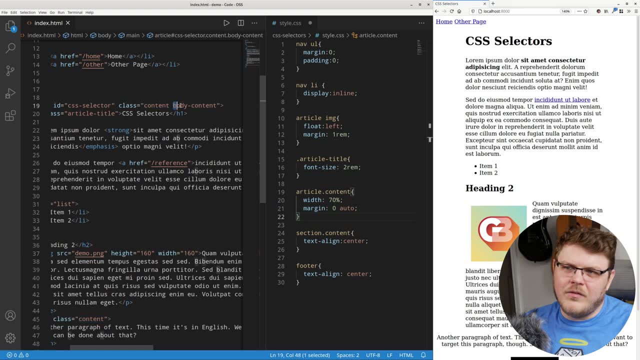 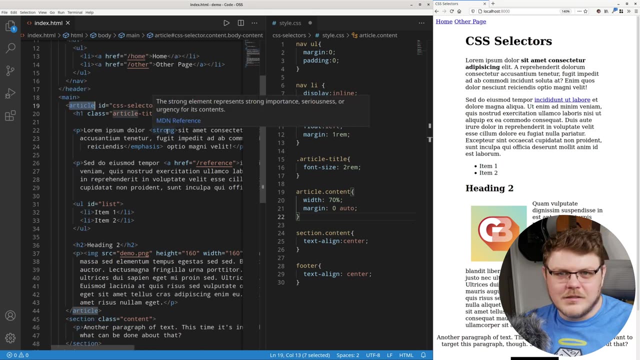 And you can see that if we refresh the page, nothing's going to change, because classes are delimited by spaces, So like, basically, you can think of content and body content as two separate entries in the articles classes. right, So there are two separate classes here. 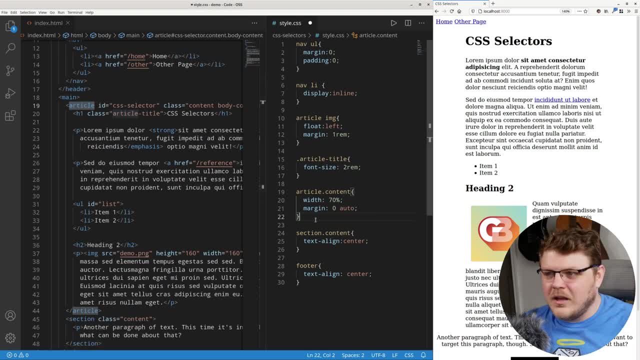 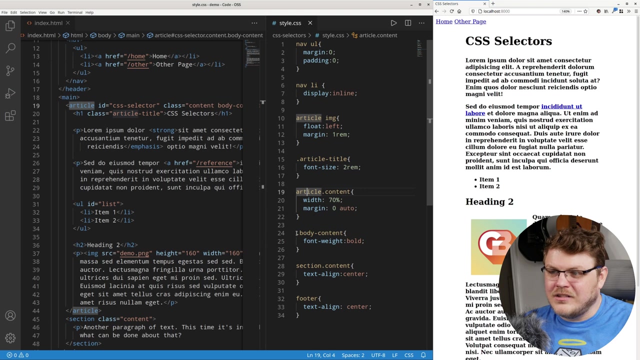 Now If you actually do different things in your CSS, you can say body content is going to equal. let's say font weight bold. And now if we refresh the page, everything's going to be bold. We're targeting article dot content and dot body content separately, but they're both. 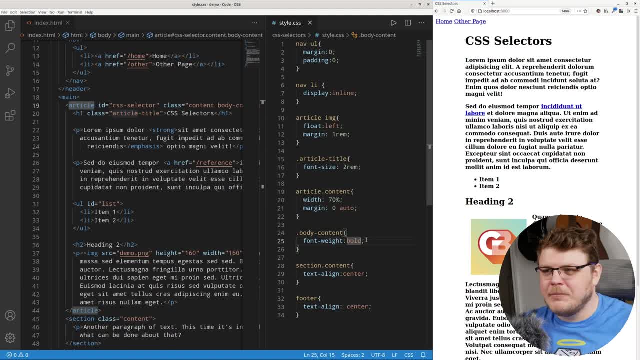 being applied to the same element. Okay, So that's a little bit tricky. So let's say we want to do a CSS selector, And this is where CSS can become a little bit tricky because you see, we also have an ID of class selector here. 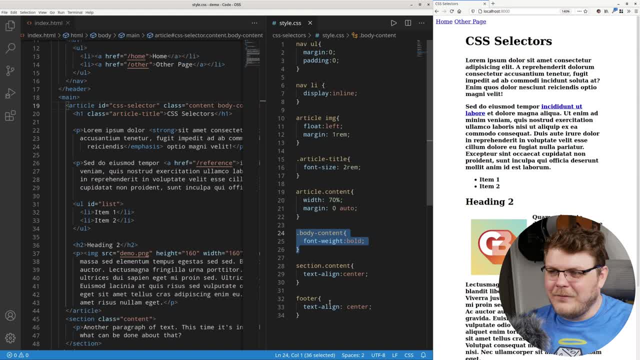 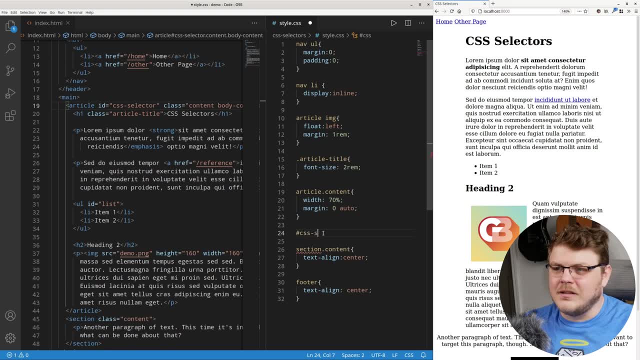 So let's get rid of this, because this is kind of ugly And we'll refresh the page Now. let's say that we want to do CSS selector. Now what does that hash mark mean? The hash is actually targeting an ID rather than a. you know. a dot for a, you know. 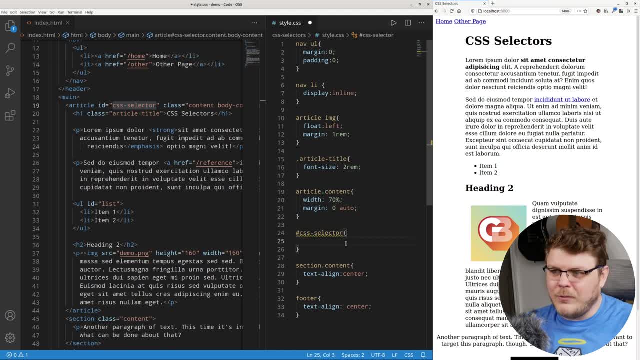 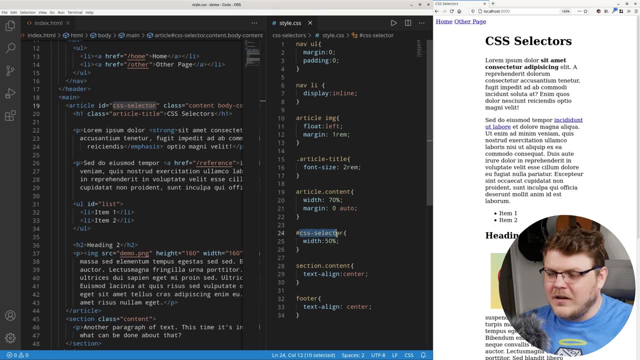 a dot for a, you know a dot, Okay, Class. And if we were to say width 50% and we leave margin and margin zero, auto, when we refresh the page you'll see that the CSS selector or the ID selector here is actually overriding. 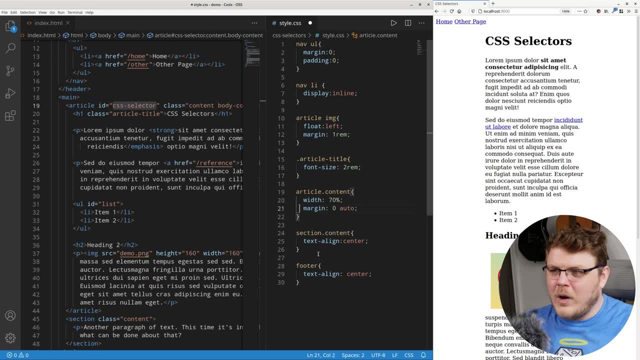 the article dot content above, And it doesn't matter where we place this. If we paste that in here, you can see that it's still taking precedence. Okay, Because, um, because an ID selector, uh, is actually going to have higher priority. 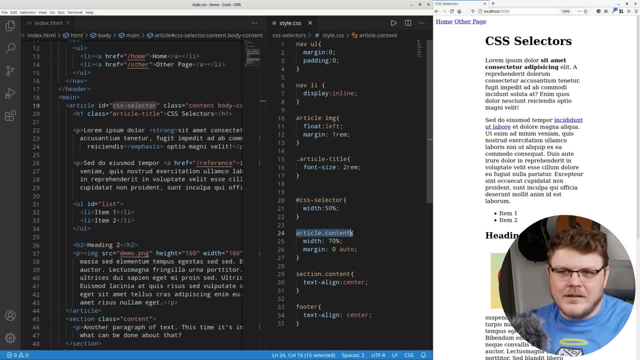 It's more specific um than an article, dot content, or even a dot content would be Um, and- and that's something that we should talk about- Uh, if we say just dot content and we say um, width is a hundred percent, and we were 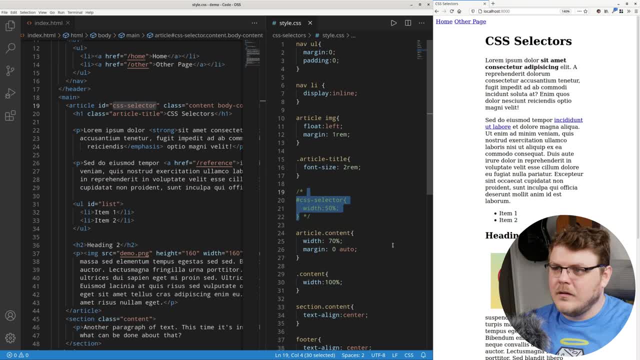 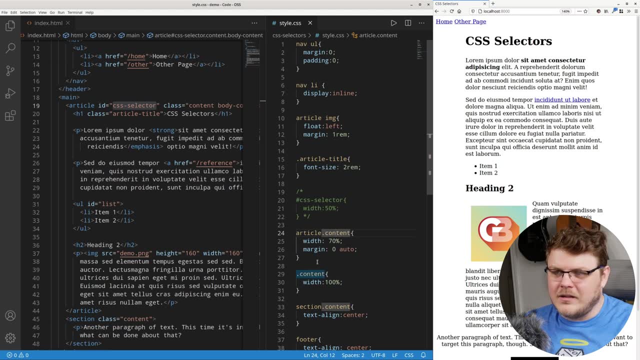 to, like you know, make this. Okay. Go away for a moment. You'll see that the article dot content is more specific than dot content, And so, because article dot content is more specific, it's going to apply its styles, Right? 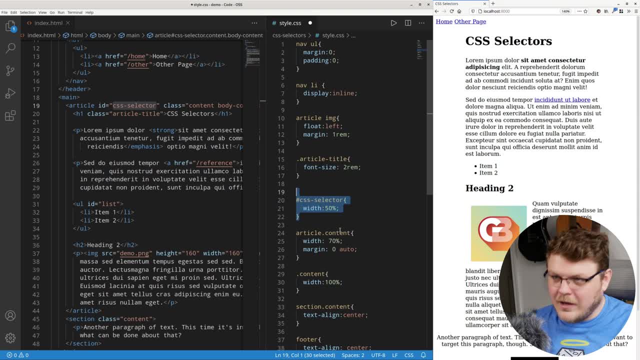 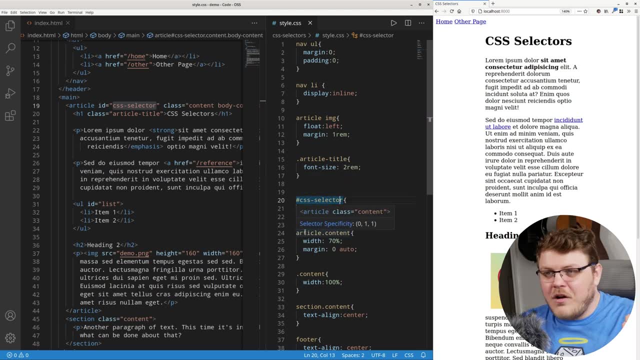 Um and again, if we uncomment that and we refresh the page, the ID tag is the most specific and then article dot content is the next most specific. Okay, That's why I'm not saying that our custom content is the last, uh, the least specific. 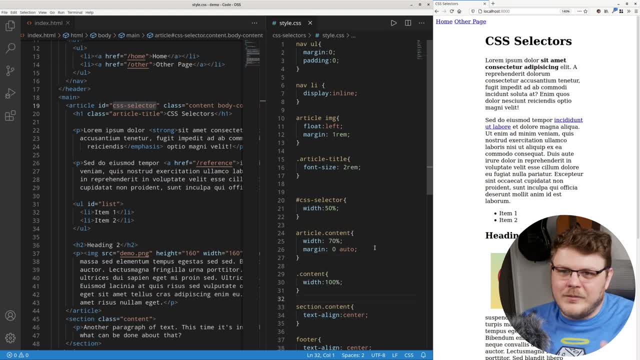 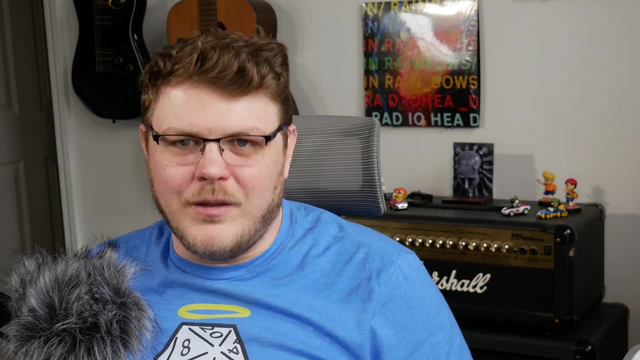 Specificity is really tricky in CSS sometimes, Um, and generally, uh, specificity of equal value is going to flow from the top of the document down, So things that are further down in the document, if it has the same specificity, uh, the, the